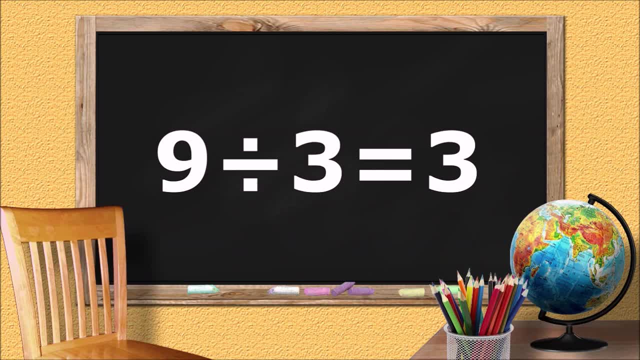 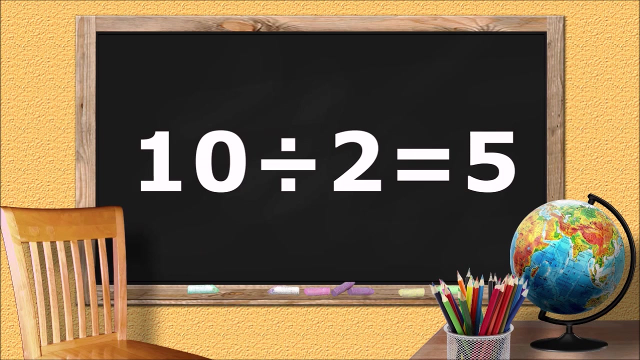 Two divided by two equals. one Ten divided by two equals. Five Twelve divided by three equals Four. Six divided by two equals. Six. Four. Six divided by four equals. One Six by four equals. One Eight divided by two equals. 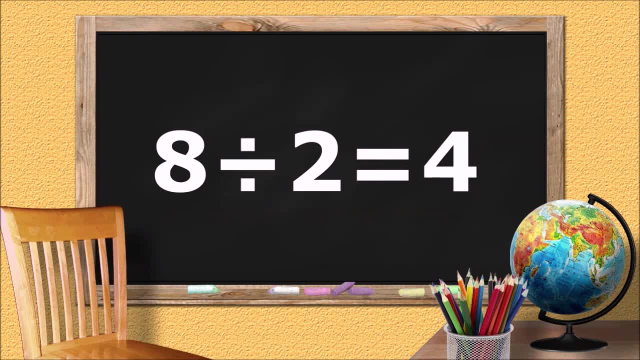 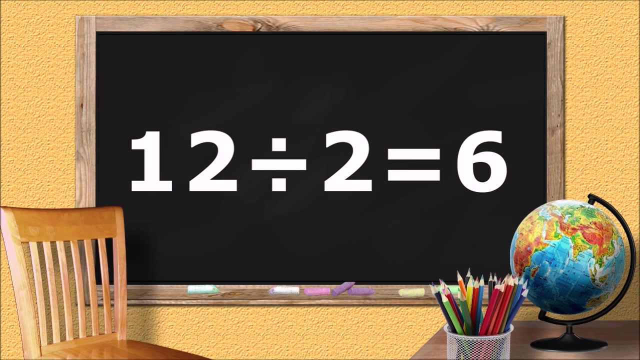 Three Eight divided by two equals. One, Four, Four, Two, 7, 20 divided by 2, equals 10, 15 divided by 3 equals. 5, 12 divided by 2, equals 6, 18 divided by 3 equals. 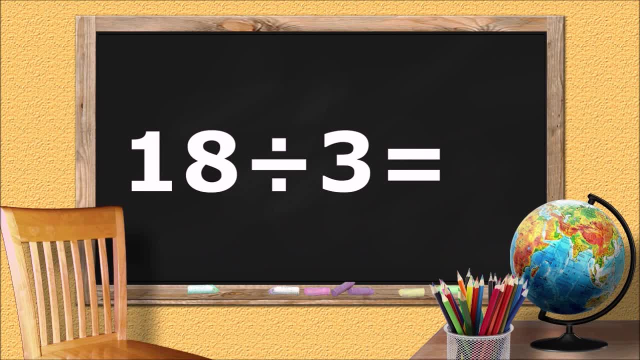 7. 6. 7 divided by 7. equals. 7 divided by 7 equals 1. 1 divided by 1 equals 1 divided by 1 equals 1. 21 divided by 3 equals 7. 12 divided by 3 equals. 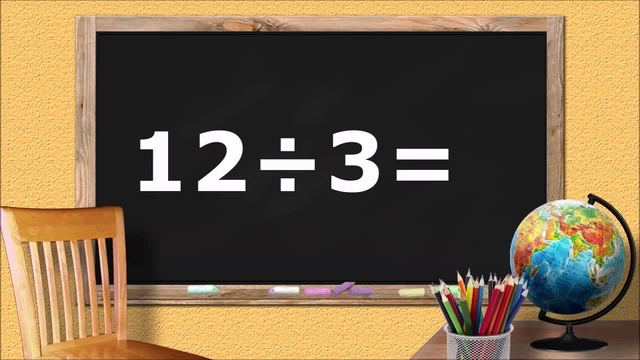 4. 18 divided by 2: equals 9. 2 divided by 1 equals 7. 2 divided by 1 equals 8. 3 divided by 2 equals 9. 3 divided by 1 equals 40 divided by 2 equals 20. 24 divided by 3 equals 8. 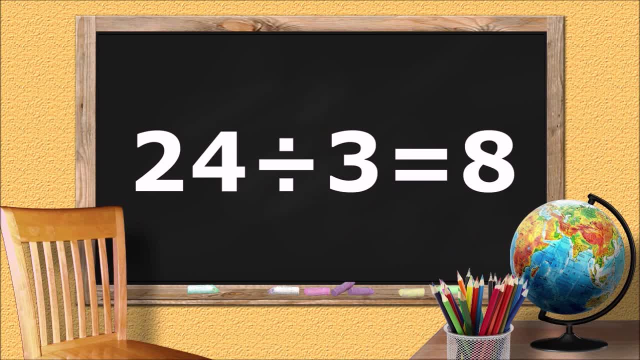 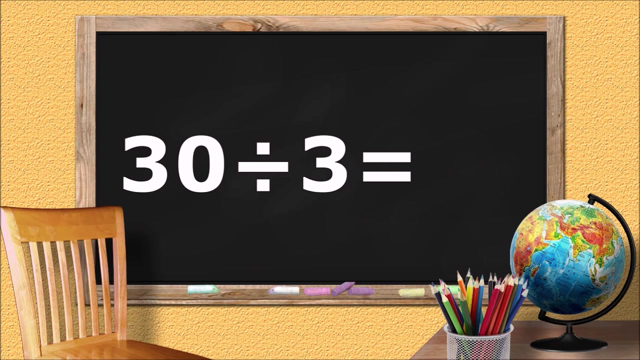